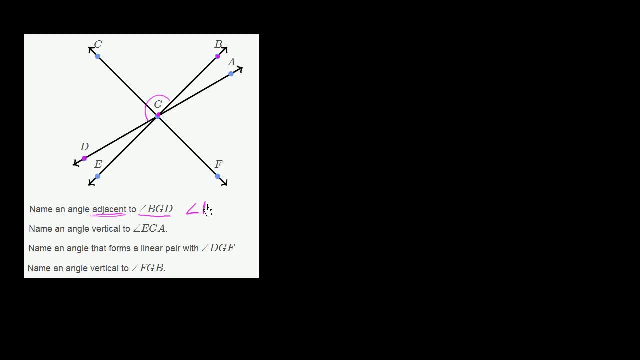 So we could say angle AGB, which could obviously also be called angle BGA. BGA and AGB are both this angle right over here. You could also go with angle FGB, because that also has GB in common. So you could go angle FGB. 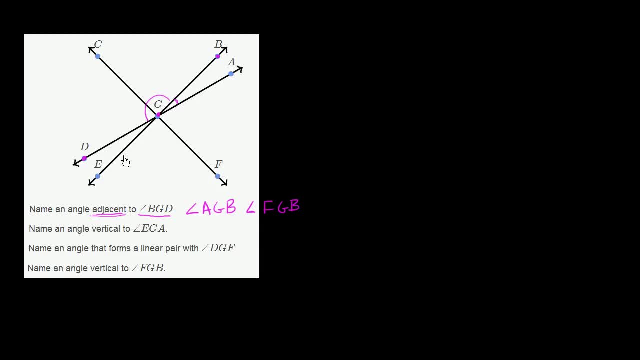 which could also be written as angle BGF. Or you could go over here: Angle EGD shares ray GD in common, So you could do this angle right over here, Angle EGD. Or you could go all the way out here: angle FGD. 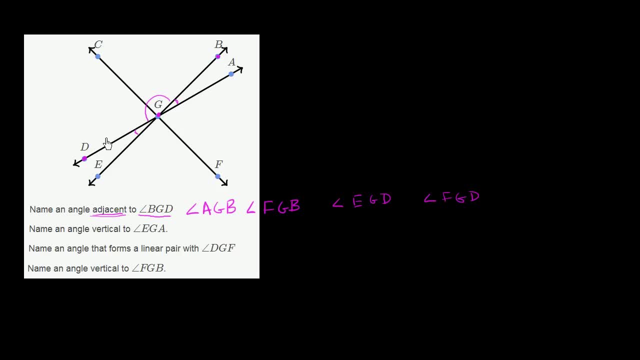 Angle FGD. These last two sharing ray GD in common, So any one of these responses would satisfy the question of just naming an angle, Just naming one. Let's do this next one: Name an angle vertical to angle EGA. Angle EGA. 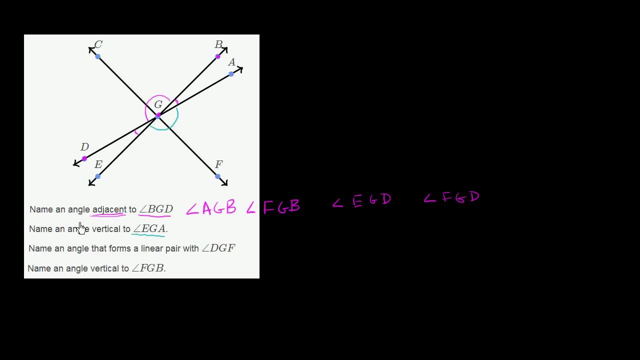 So this is this angle, This is this angle right over here, And the way you think about vertical angles is: imagine two lines crossing. So imagine two lines crossing just like this, And they could literally be lines And they're intersecting at a point. 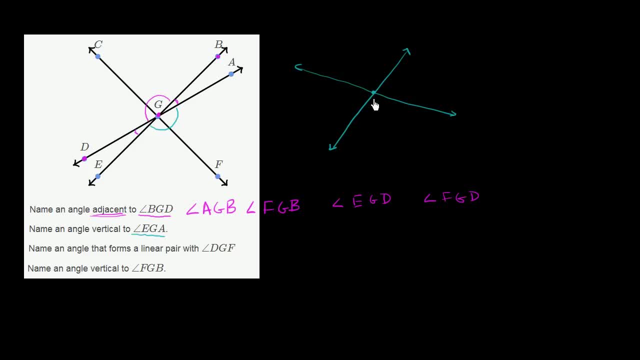 intersecting at a point. This is forming four angles, or you could imagine it's forming two sets of vertical angles. So if this is the angle that you care about, its vertical angle is the one on the opposite side of the intersection. It's one of these angles that it is not adjacent to. 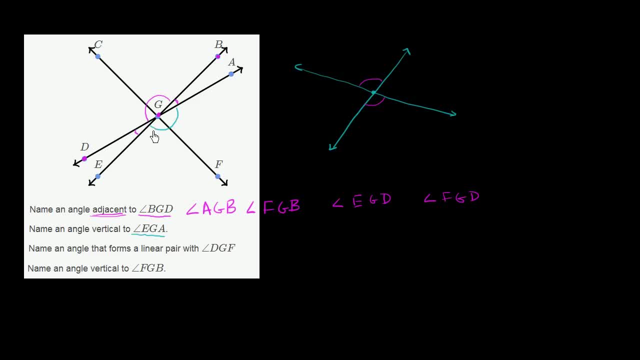 So it would be this angle right over here. So, going back to the question, a vertical angle to angle EGA. well, if you imagine the intersection of line EB and line DA, then the non-adjacent angle formed to angle EGA is angle DGB actually. 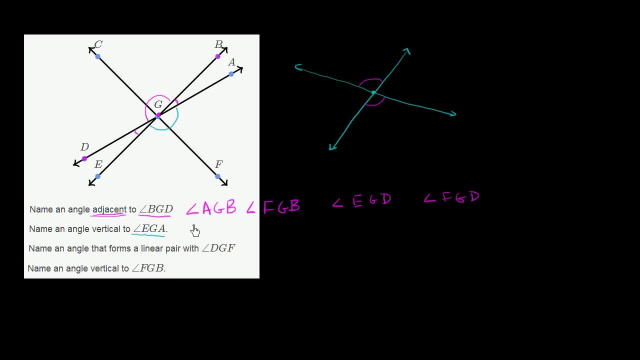 what we already highlighted in magenta, right over here. So this is angle DGB, which could also be called angle BGD. These are obviously both referring to this angle up here. Name an angle that forms a linear pair with angle DFG. 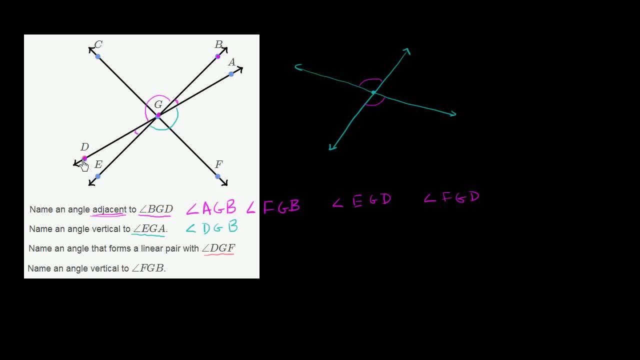 So I'm just in a new color Angle: DGB, D-F-G, D-F- Oh, sorry, D-G-F. All of these should have G in the middle, D-G-F, So linear pair with angle D-G-F.